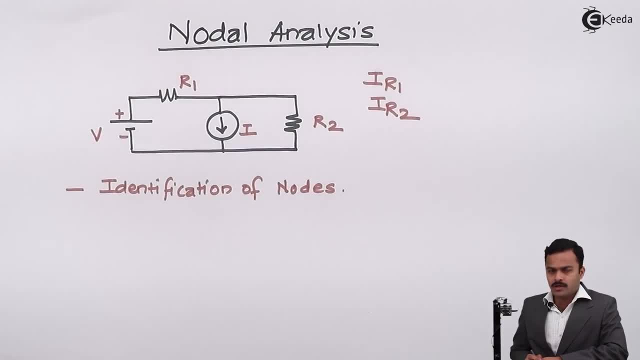 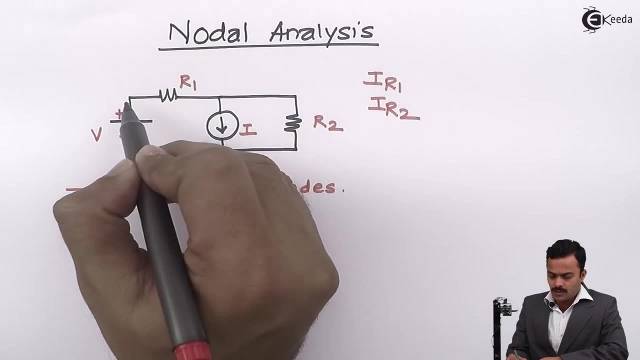 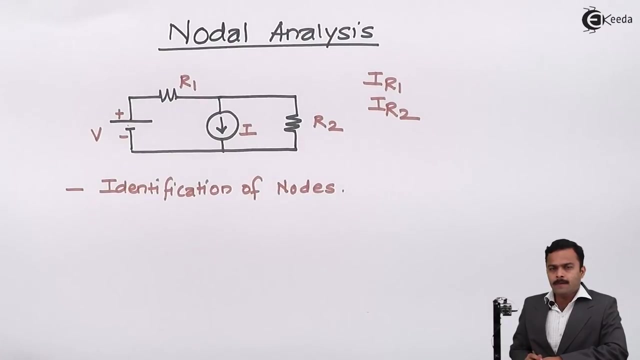 more than two branches are connected. So I repeat, node is a point or a junction where more than two branches are connected. So I cannot consider this as a node for nodal analysis, because 1 and 2. branch means the number of elements present between two nodes. 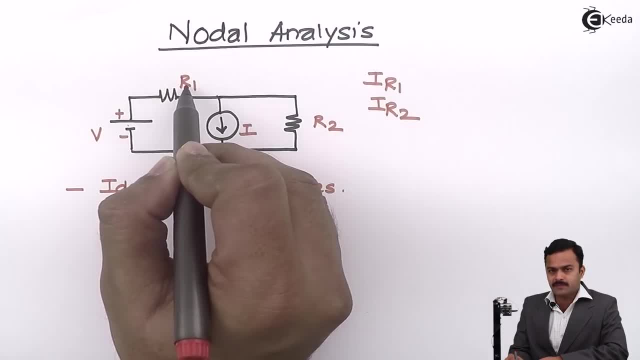 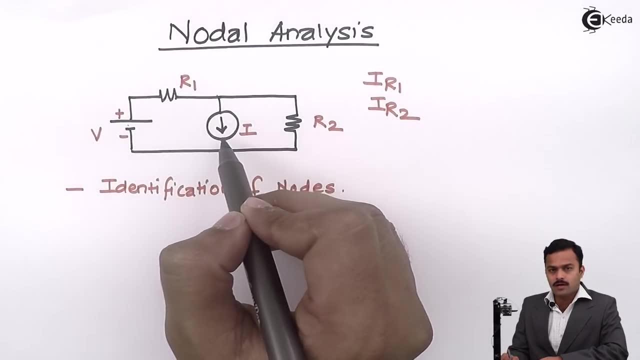 So I can say this is also a branch because of the element is present, that is, resistance. This is also a branch because of the element voltage source is present. This is also a branch. current source is present. This is a branch where resistance is present. 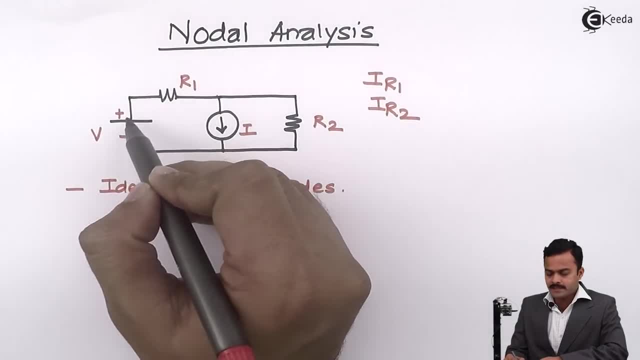 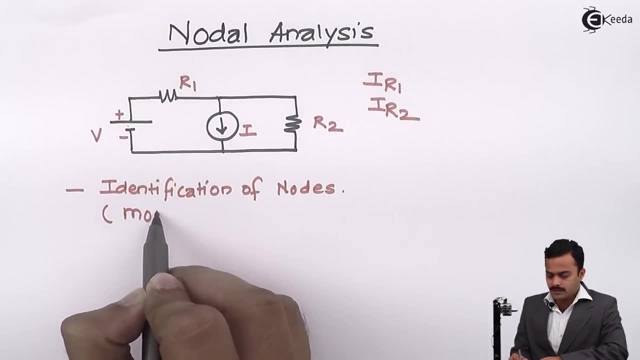 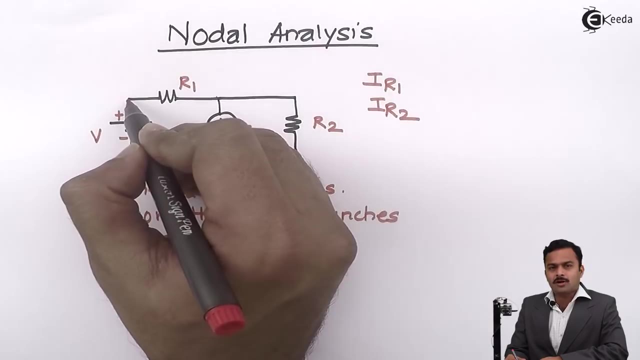 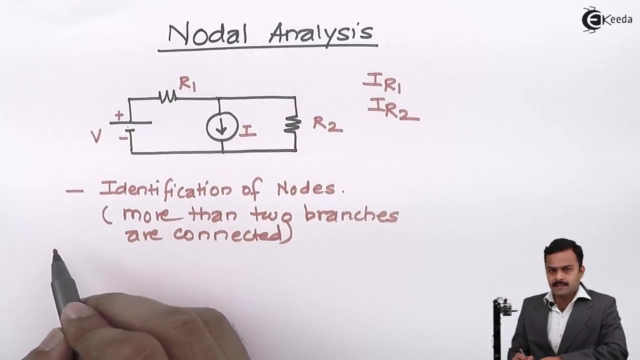 R2 is present. now, here two branches are connected. but here what we are saying node is nothing but a point where more than two branches are connected. so this cannot be a node for me. this point, one, two, three, three branches are connected. yes, so this will be a significant node, so I will name it as VA directly. I name: 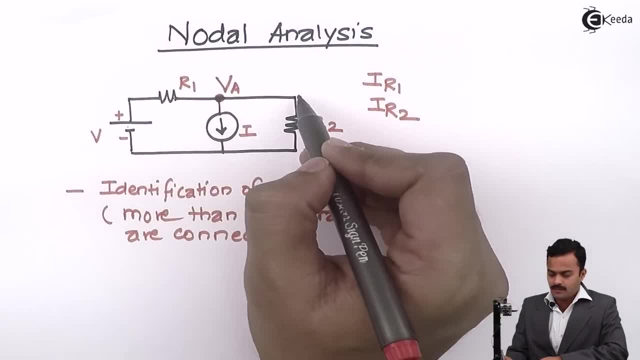 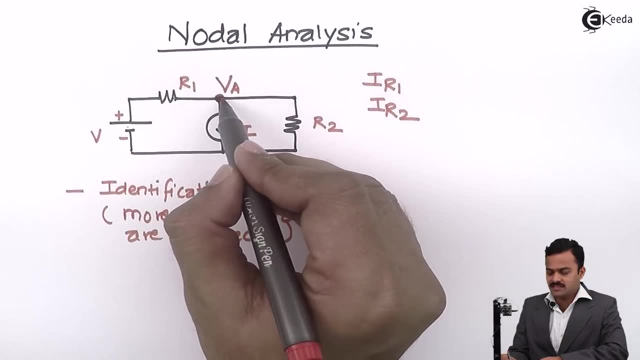 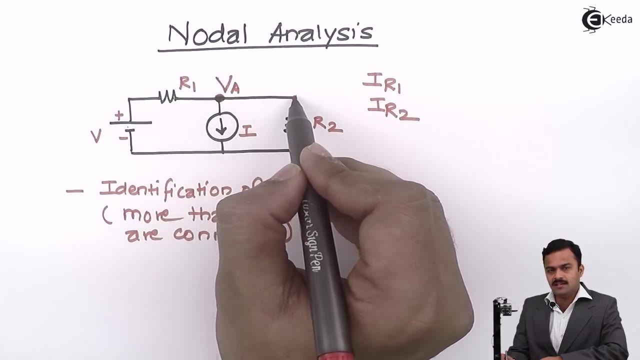 a potential of this node is VA. this cannot be a node, because two branches, rather this cannot be a branch for me because it's just a wire, just a line. there is no element present between these two point, so I cannot consider this as a branch. so here I have only one branch, that is. 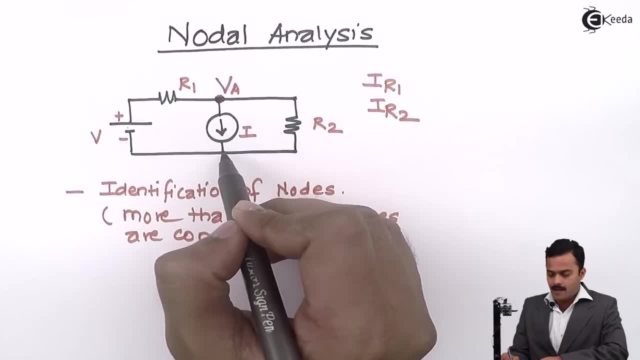 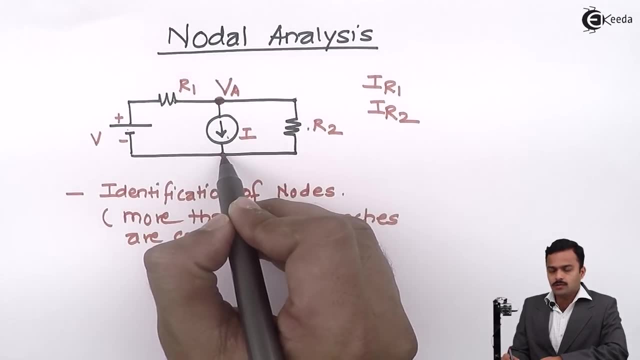 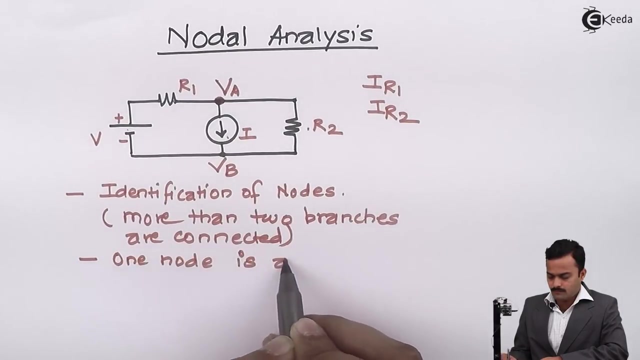 R2.0 till this point, and at this point I am having one, two, three branches connected, so this is also another significant node. so I will mention it as VB. once you identify how many nodes, are there one node you have to take as a reference. reference means I will take voltage. 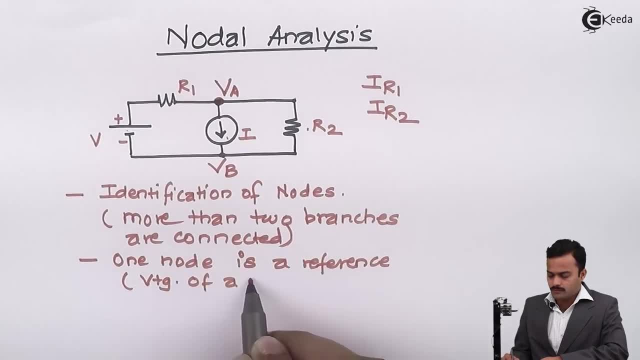 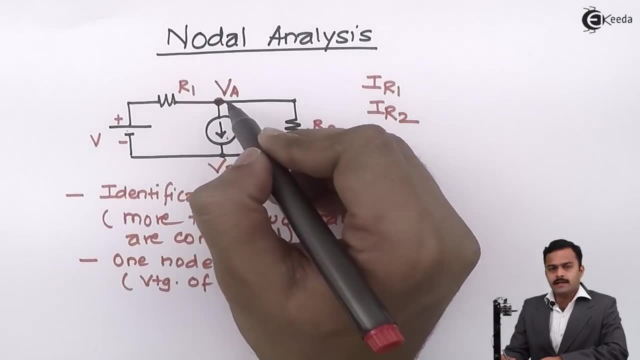 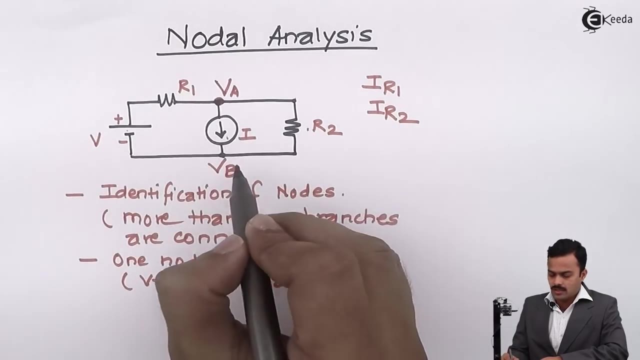 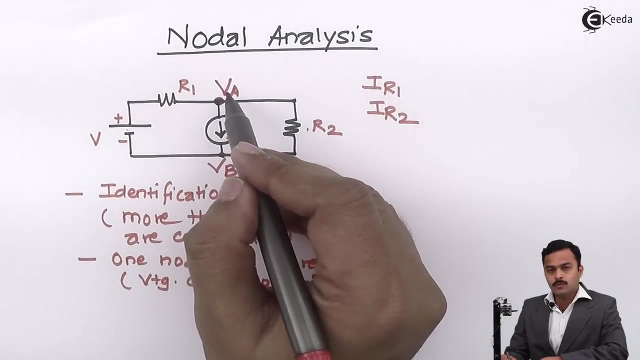 voltage of that node is zero. so in this particular circuit I got two nodes. one of the nodes I have to take as a reference, so I will take this node as a reference- means the potential of that node I will take as zero. so I will have only one significant node. so I have to get a voltage of that node, which I have. 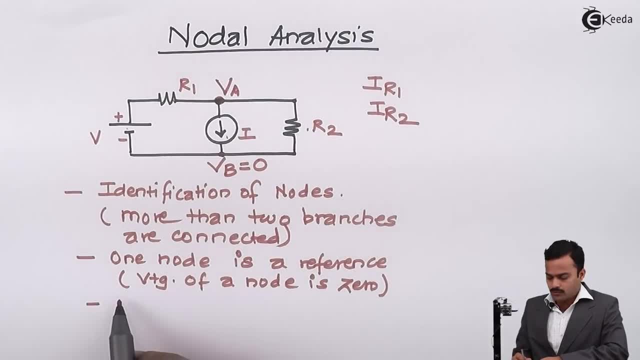 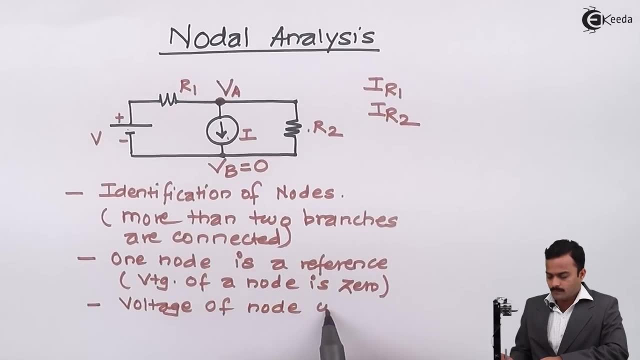 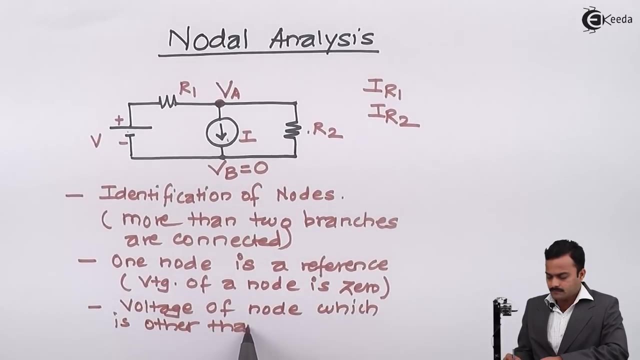 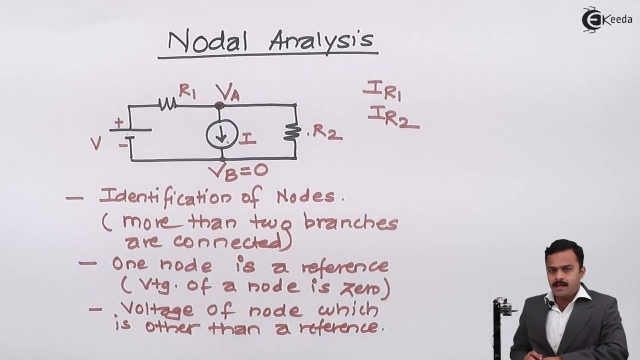 not taken as a reference. so here I have to calculate voltage of node, which is other than a reference in this problem. it is VA. so this is the problem and the other problem is VA, and once VA is known I can get all the branch currents. how to get branch? 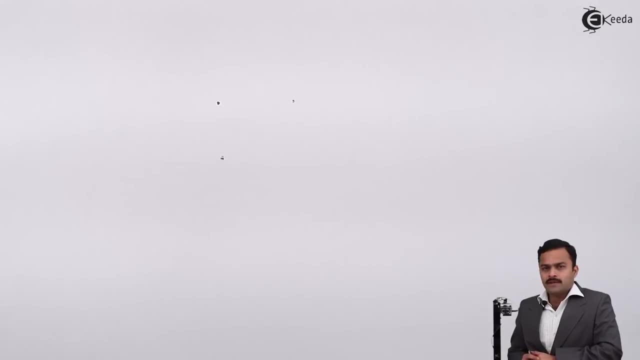 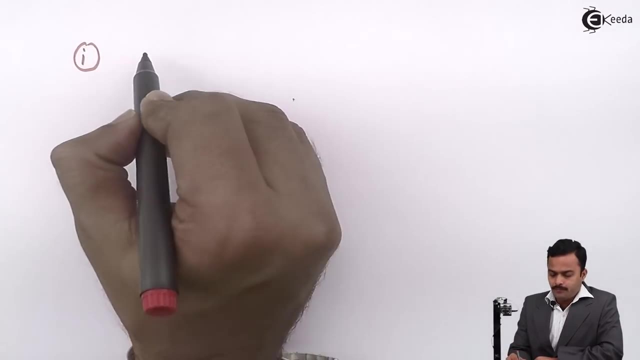 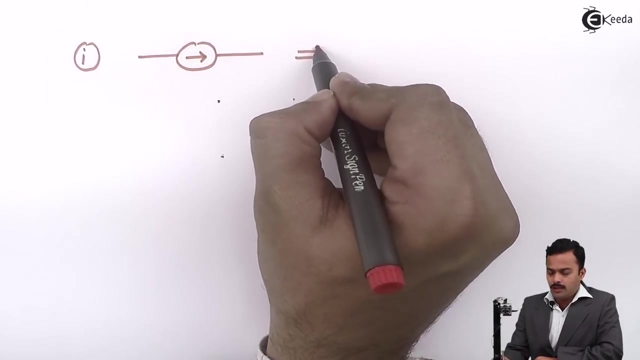 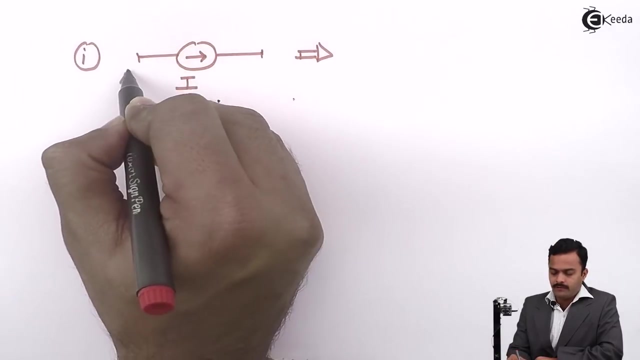 currents. for this purpose, let's have three simple techniques. so technique number one: if branch consists of a current source, then simply the value of this current source, which I will take as, say I, which will be branch current between point A and B. so I will mention here points A and B, where current source 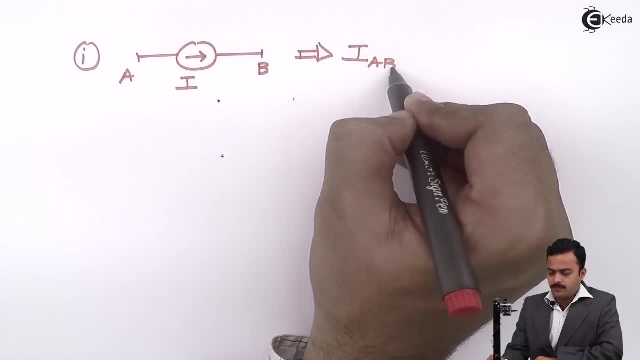 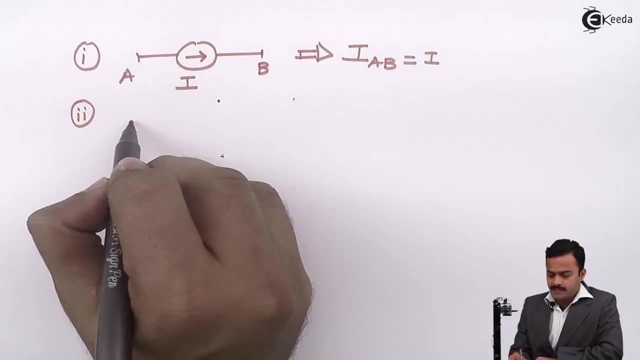 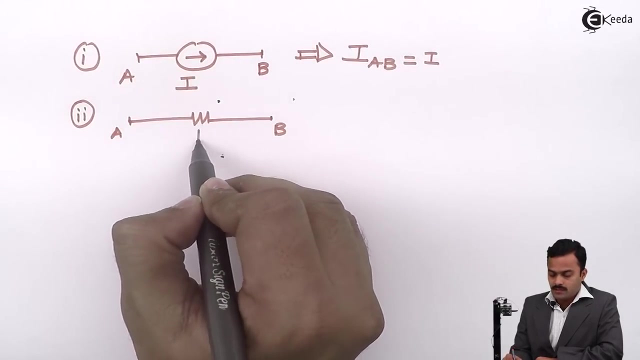 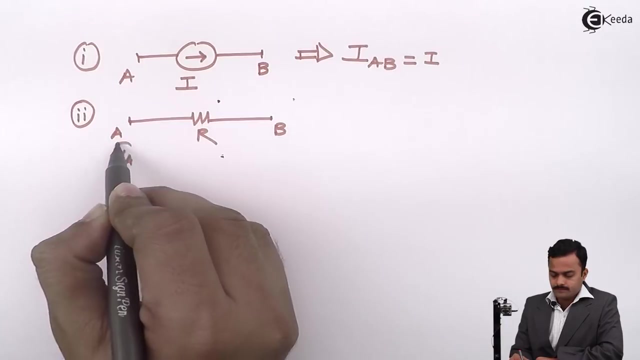 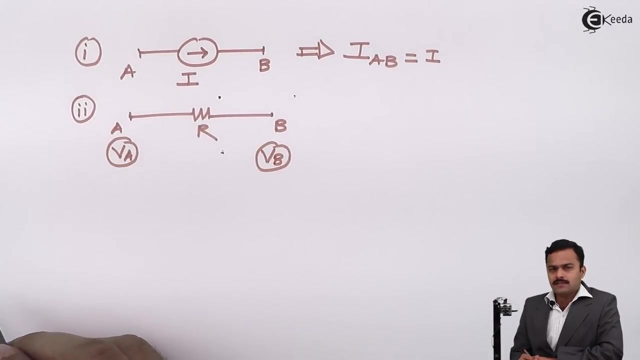 is present. so I can say current flowing through the branch IAB is. I second suppose there is a resistance between two points or two nodes having the value R, now the node potential of this, a point, its VA, more potential of this V is VB and based on the direction of current that we have chosen. so, for example, I 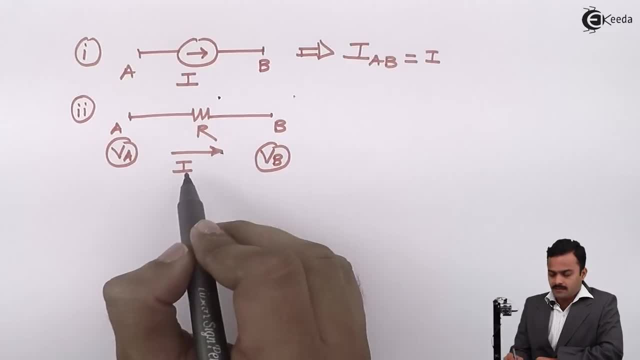 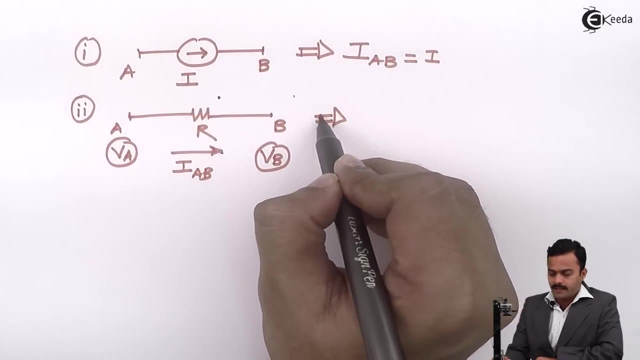 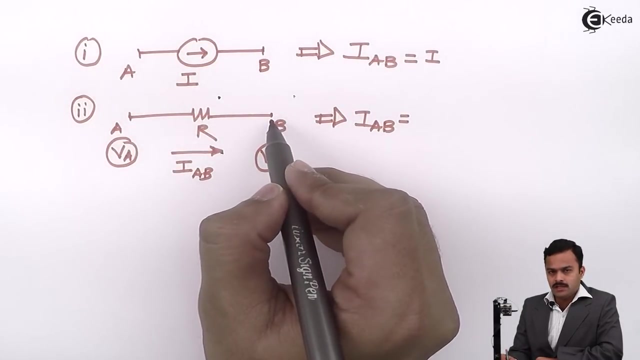 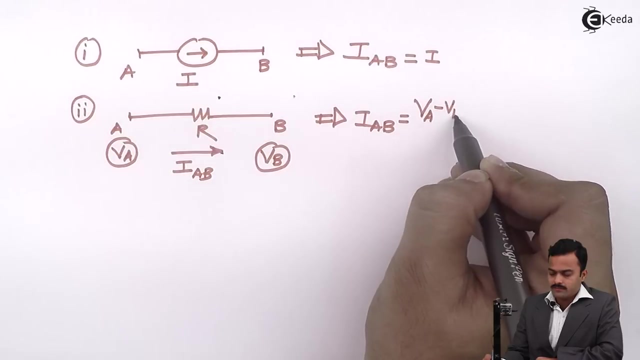 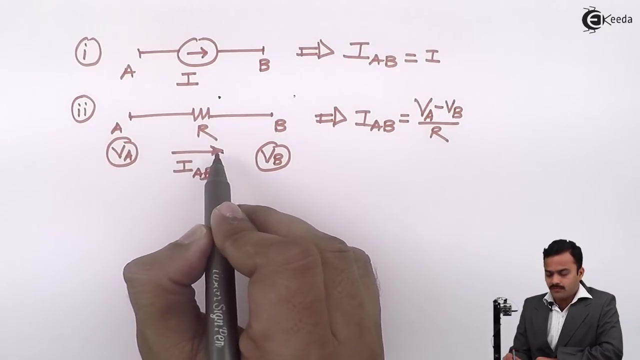 have consider current like this: I, which I will mention as IAB, from A to B, so I can write the equation: current, flowing through this branch, is nothing but the but potential difference between these two points divided by resistance. so potential difference is VA minus VB upon R. see, it depends upon the direction of 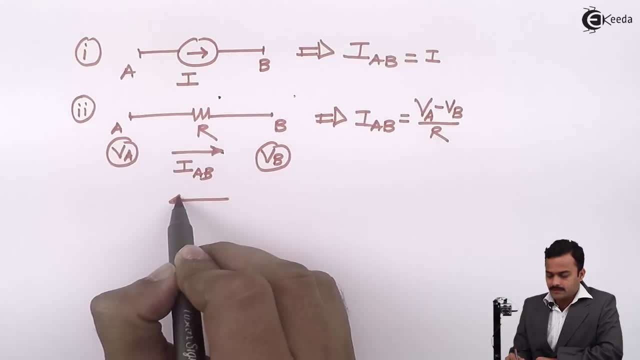 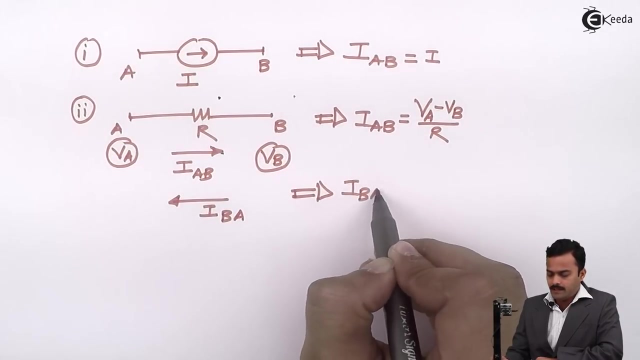 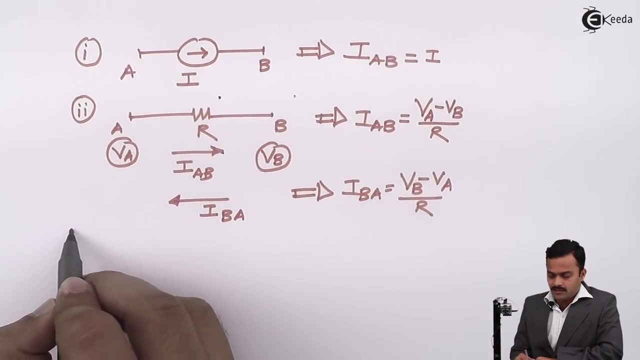 current meaning, suppose I take a direction like this, which I will mention IPA. so here I have considered: B is at higher potential compared to a, so I be a equals VB minus VA divided by R. so, based on the direction that we have selected as per that, this equation will change. and third, most important rule: 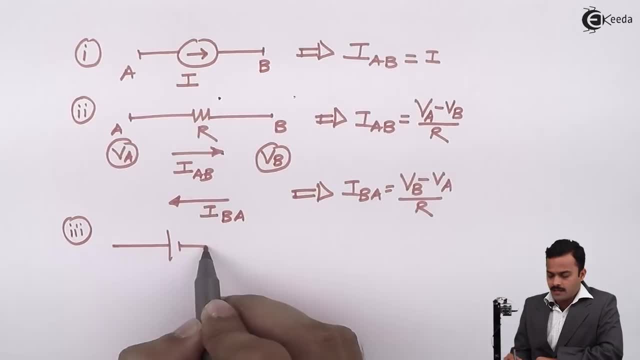 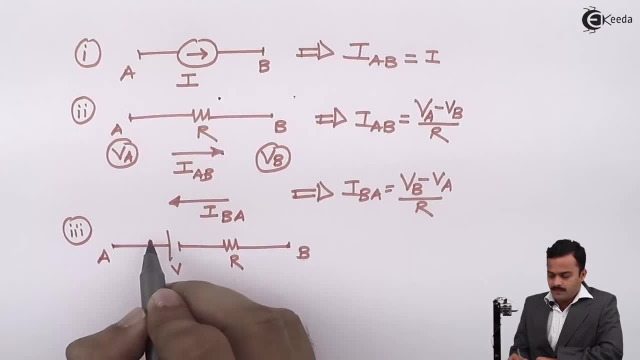 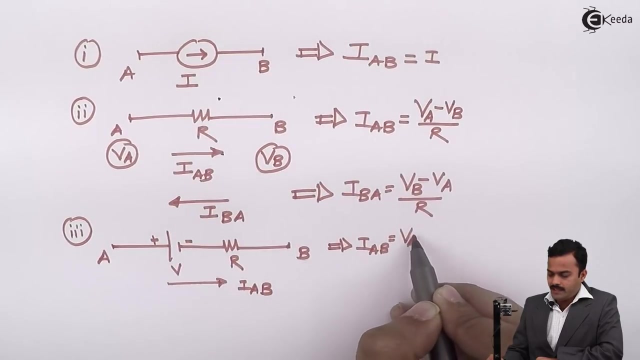 voltage B. this is the resistance R and polarity, as I mentioned, and suppose I am considering current direction like this. so the equation we will get, as since I consider current flowing from a to b, so obviously i am considering va is at higher potential compared to vb, so va. 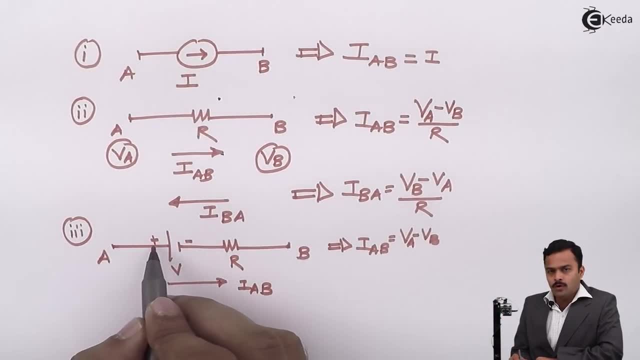 minus vb obviously there. but one more voltage source is there. so in the direction of current, which is a to b, i am having voltage polarity changing plus to minus, so initially it is plus, now it has become minus in the direction of current. so there is voltage drop, so it is minus. 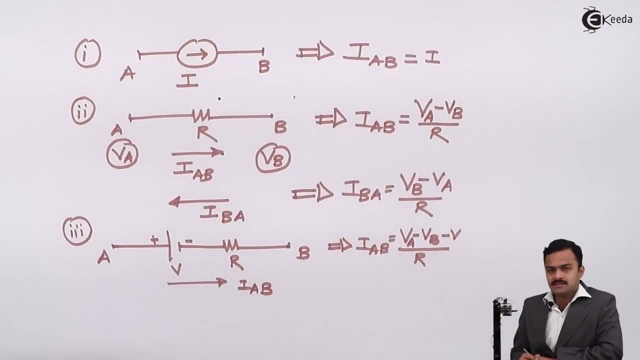 v divided by total resistance in a branch. suppose i will consider current direction like this. so i will get a equation: iba equals. now, current direction is from b to a, so i assume it Indirectly B has higher potential compared to A. so VB minus VA. and in the direction of current, which is from B to A, I have voltage polarity changing minus to plus. that means initially it is minus, in a current direction it has become plus. 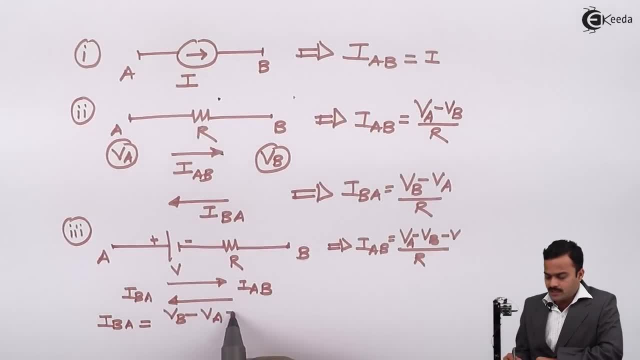 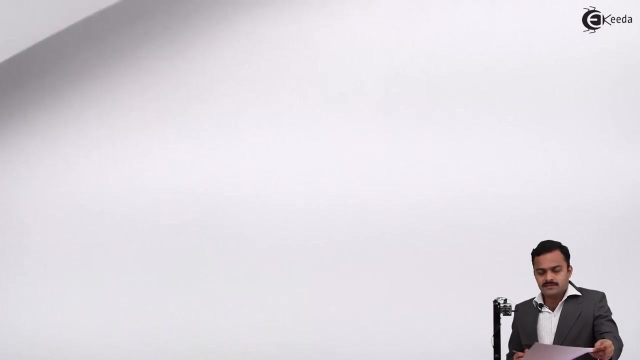 So there is voltage rise. voltage rise I mentioned as plus plus V, divided by total resistance in a circuit from B to A, which is R. So, keeping these three techniques in mind, we can write the equations for the circuit that we have selected. So let's go back to the circuit once again. So I have this circuit now. 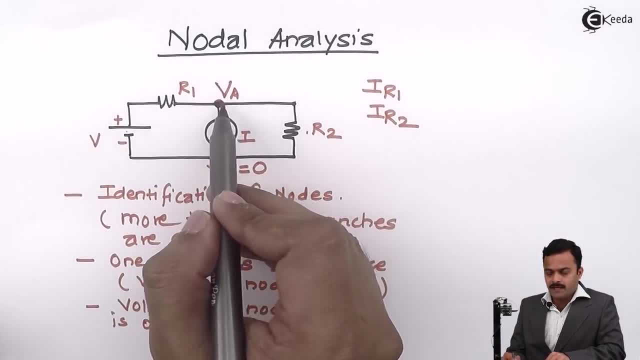 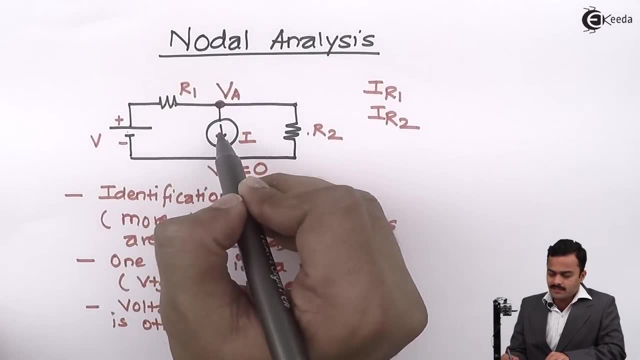 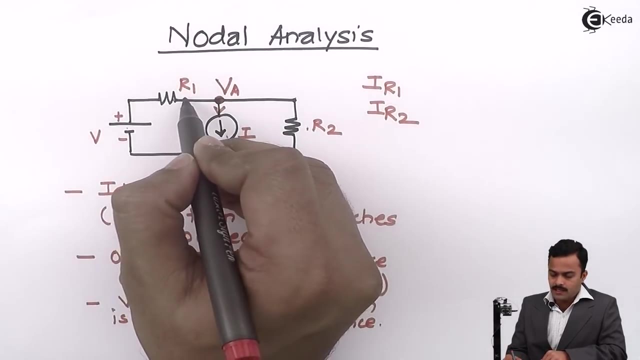 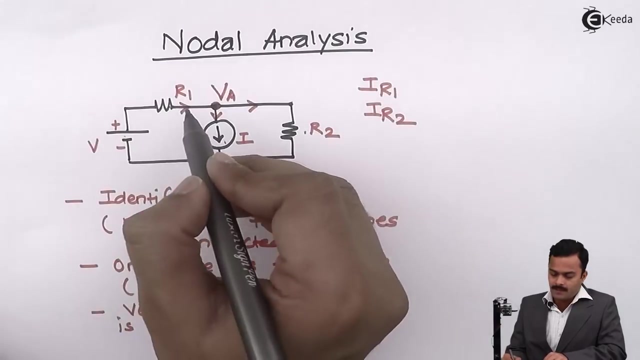 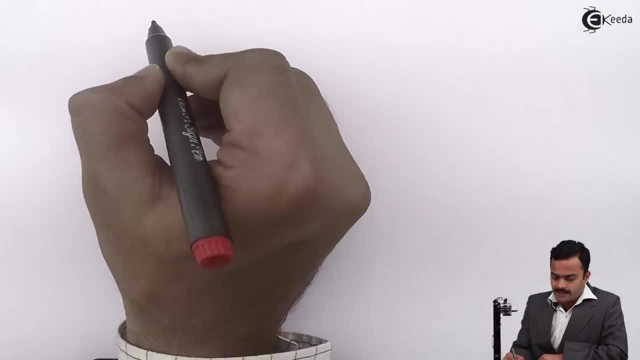 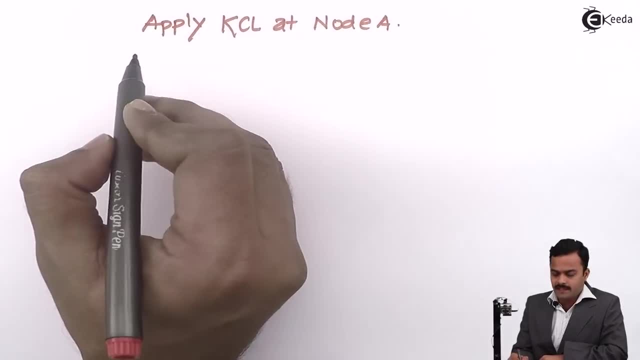 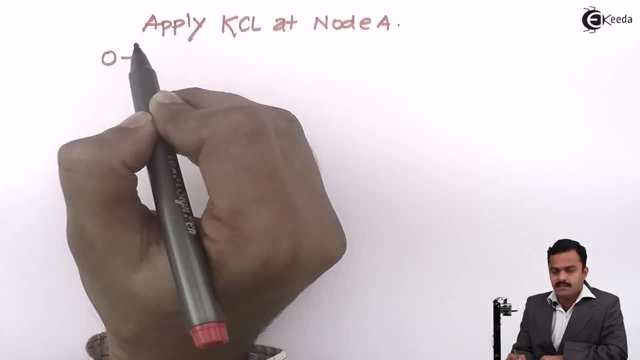 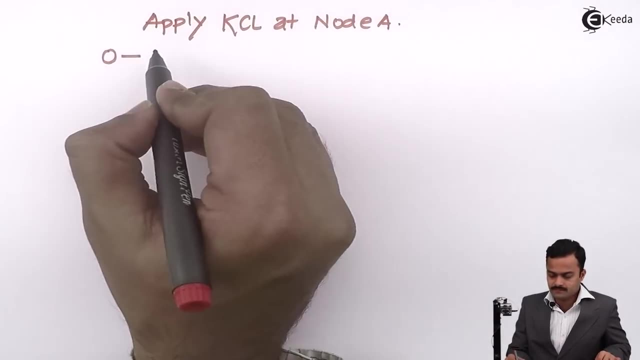 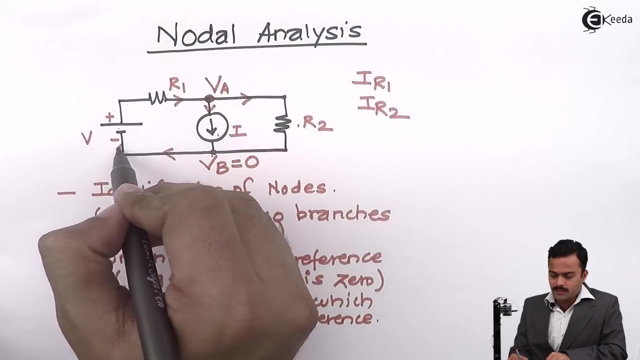 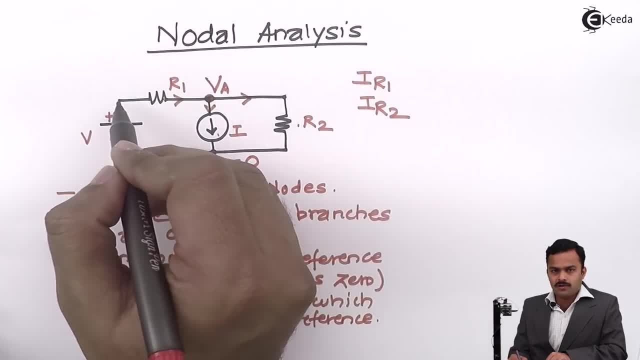 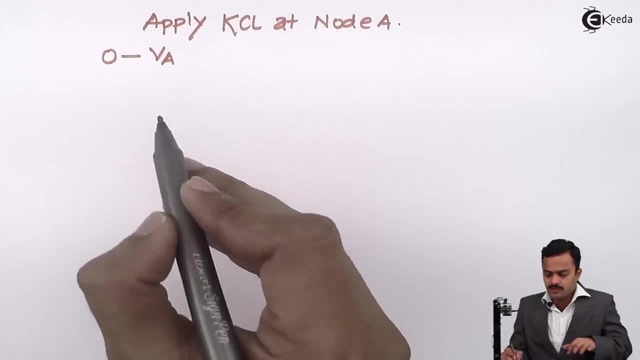 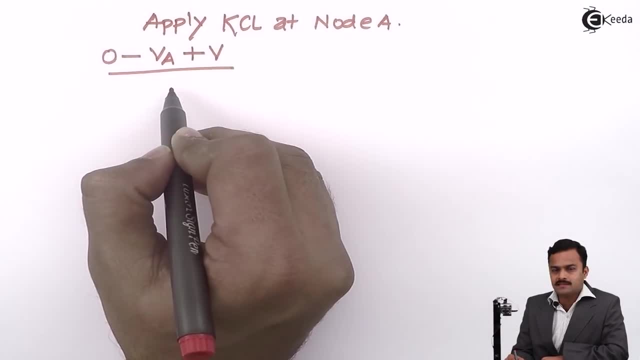 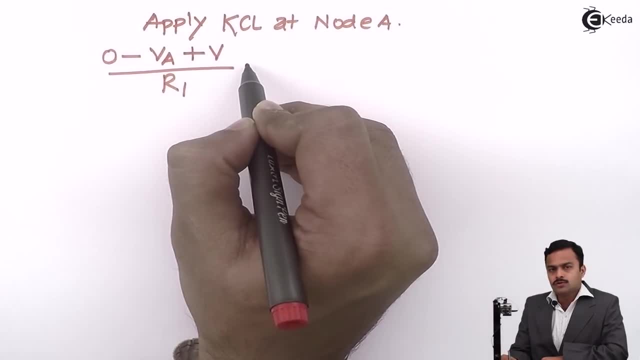 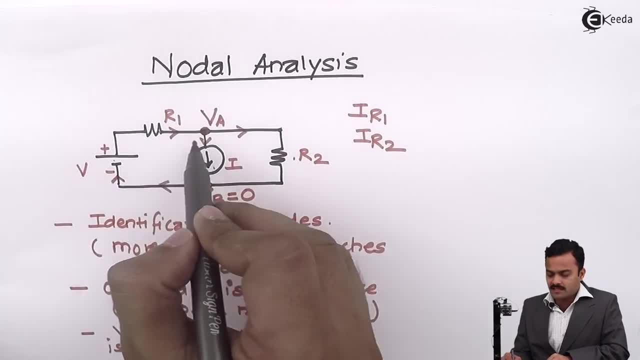 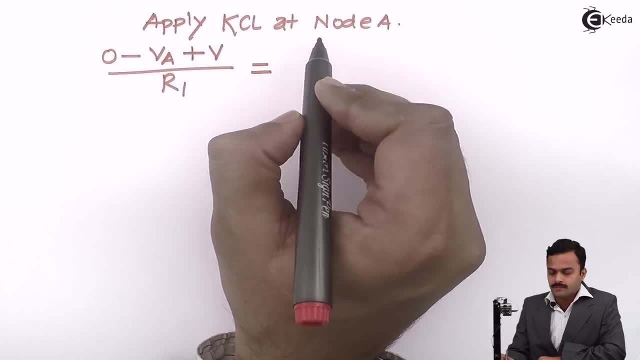 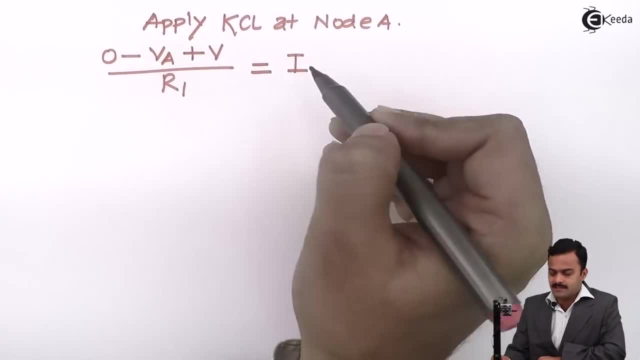 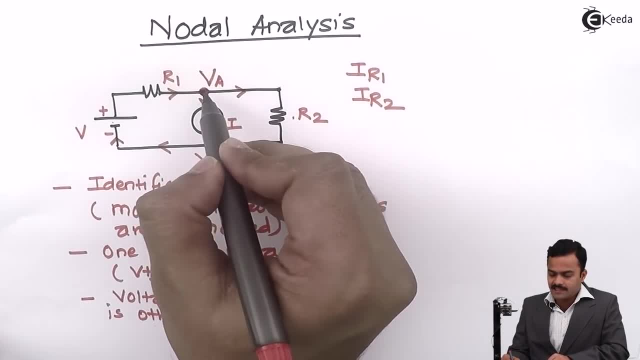 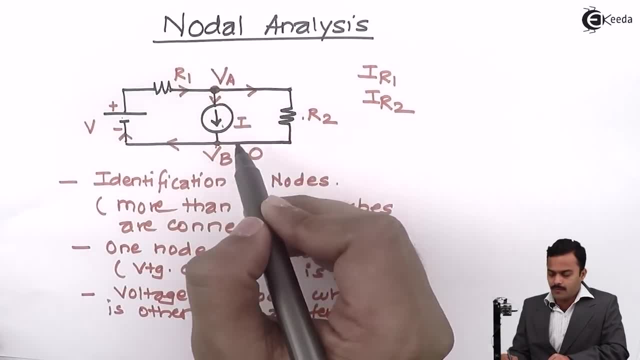 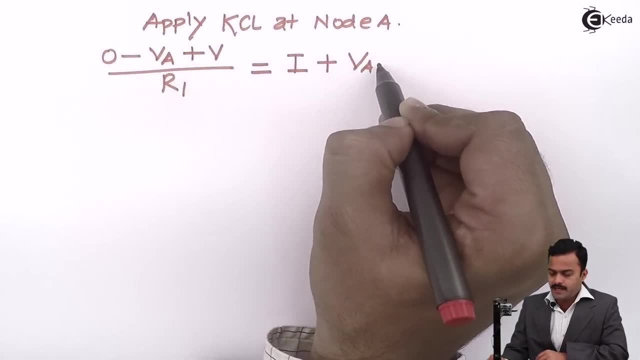 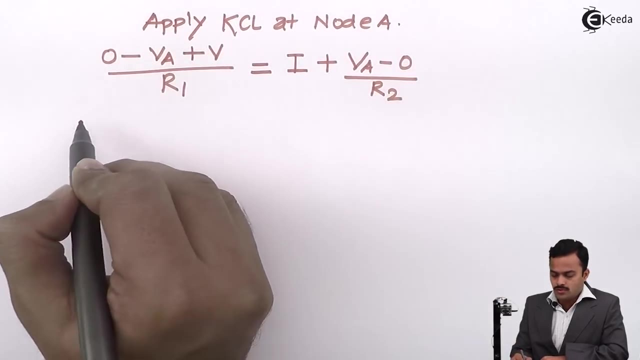 So from reference, it has started from the reference. So, from reference, it has started from the reference. So, from reference, it has started from the reference compared to B as far as potentials are concerned. so I can write VA minus 0 divided by resistance in this branch, which is R2. so here I am having only one. 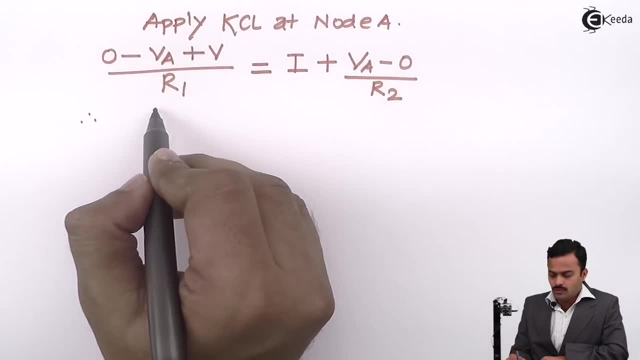 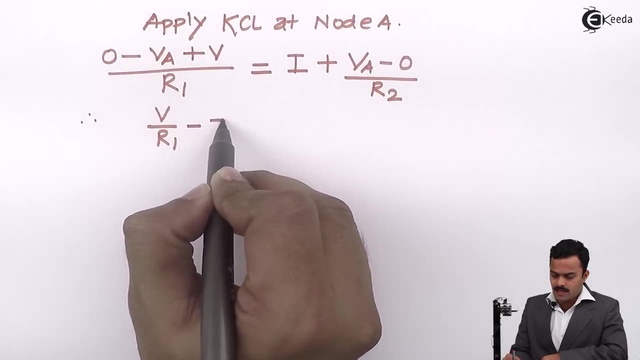 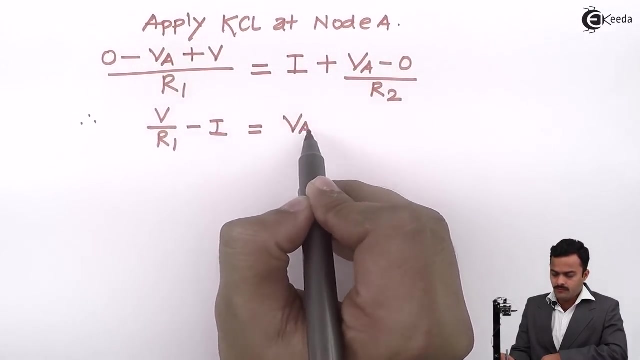 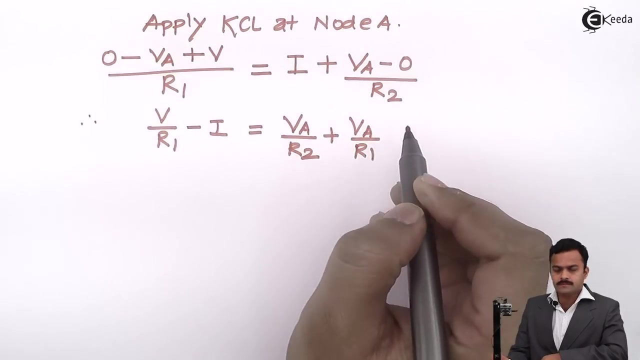 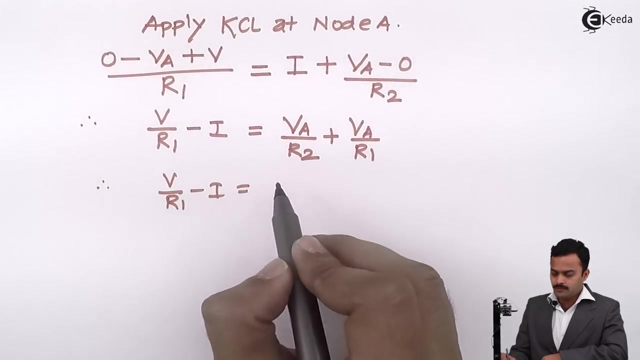 unknown potential, that is VA. so I will rewrite the terms: V by R1 will be the fix minus I- again a fix and I can take to this side equals VA upon R2 plus VA upon R1. so this term I will get as a fixed value. VA is the only unknown. 1. 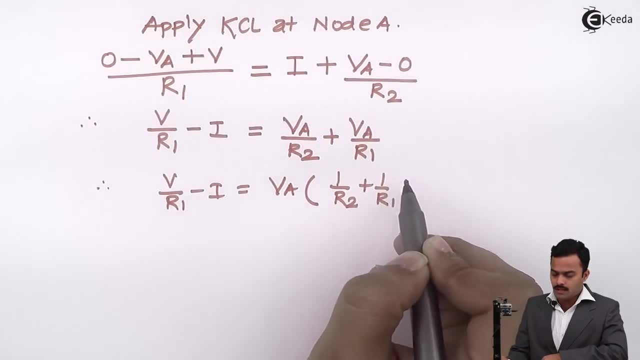 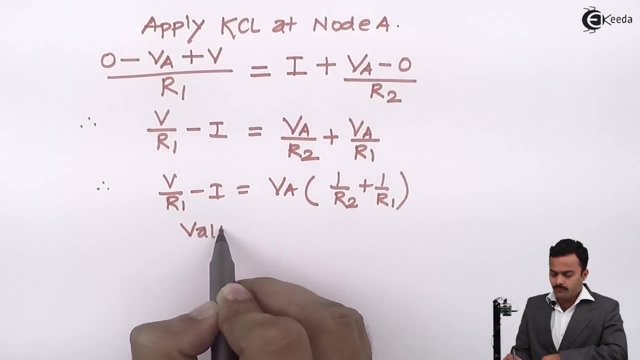 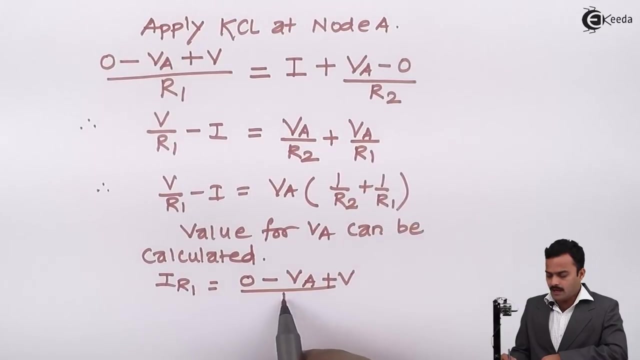 upon R2 plus 1 upon R1. R1- it's also fixed, so from this I can get value for VA once a potential of a node is obtained. I can get any branch term, meaning current, flowing through R1 I can get as 0 minus VA plus V divided by R1. 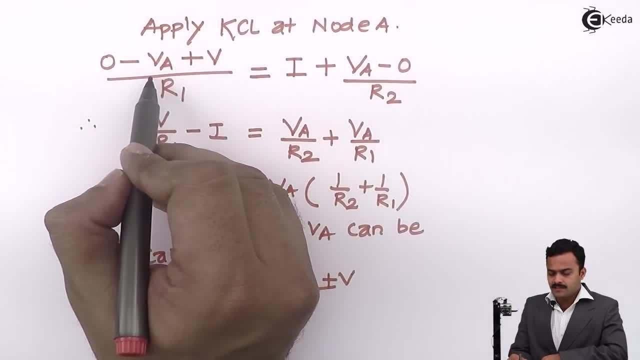 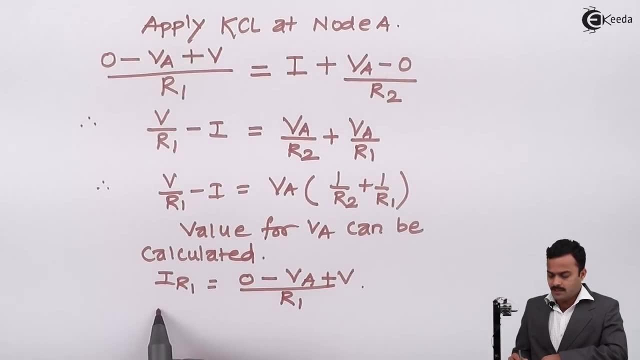 because this was a time which was telling. it is a current flowing through R1, so substituting the value of VA, I can get IR1. similarly, substituting the value of VA in this equation or in this cell, I will get VA minus 0 divided by R2. if I substitute VA, I will get IR2. so here we.